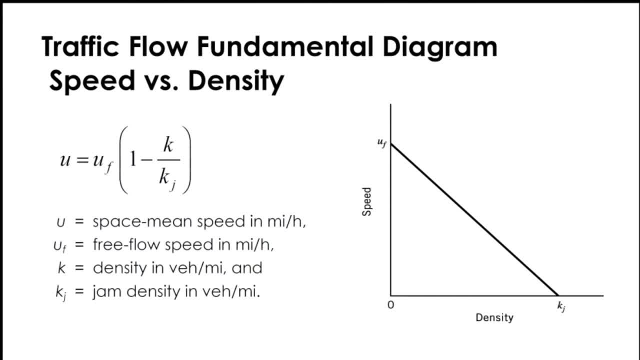 which, again, it's very simple: It assumes a linear relationship between speed and density. Today, because of the amount, because of a lot of real data that we have access to, we know that this is not necessarily the case. The relationship between the speed- density is not really exactly linear. But again, it's a model. 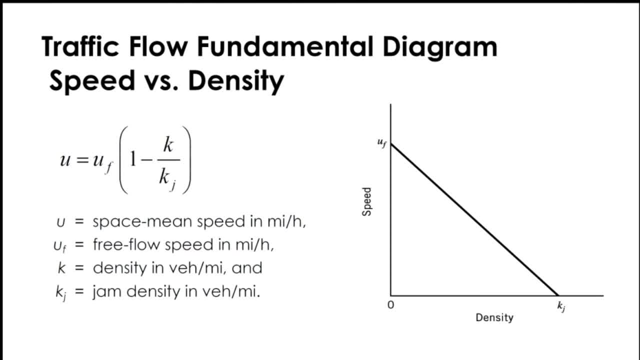 It has some, it has its own properties, It has its own advantages and disadvantages, And it's an approximate of that relationship, as I said. So here, let me find my pen. actually I wanted to draw on the. okay, I found my pen. Yes, So U represents a speed, So Y-axis is U, UF is the free flow speed. 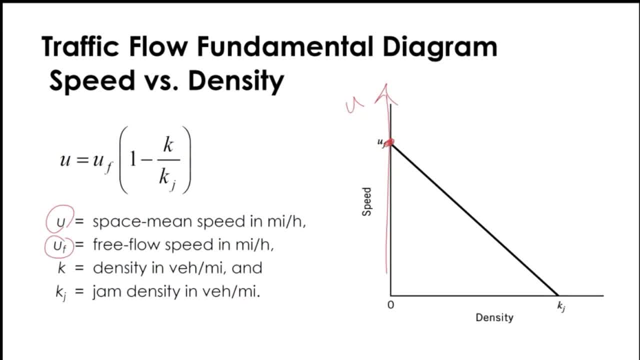 It's this point where the density is zero, speed is maximum. K represents density and it's shown on the X-axis, And KJ is jam density, which is basically the maximum density we can get when the speed is zero, when traffic is, when traffic is actually at the gridlock level and no one- everyone is. 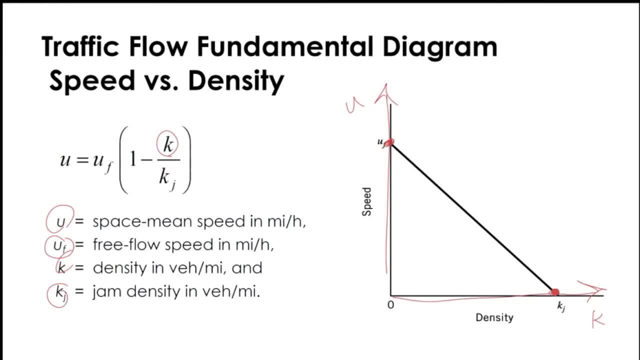 everyone's stopped what would be the maximum density? So that's KJ. So this formula is basically the equation for this line, with the intercept of UF on the Y-axis and an intercept of KJ on the X-axis, So U would be UF one minus K over KJ. This is also called Green-Shields model. 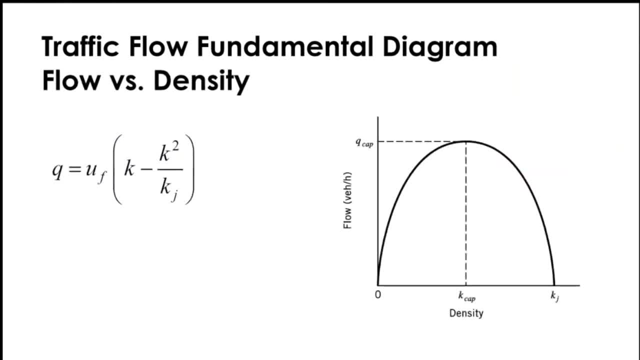 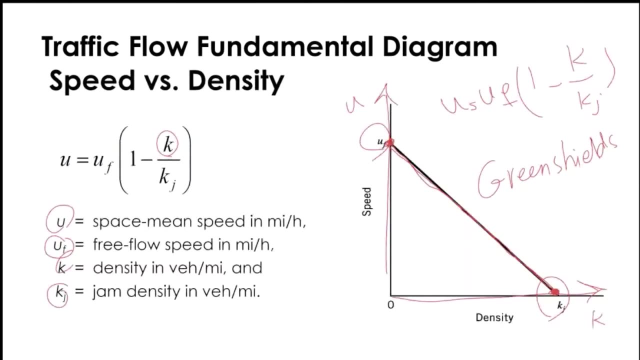 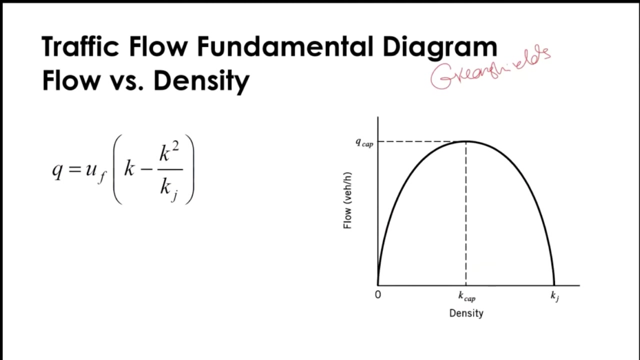 We can also derive an equation for flow density relationship. This is also called Green-Shields model. All of this models that I'm now showing you are Green-Shields model, So very similar to the linear relationship that we had for speed density. we can also derive a parabolic type relationship for flow density. 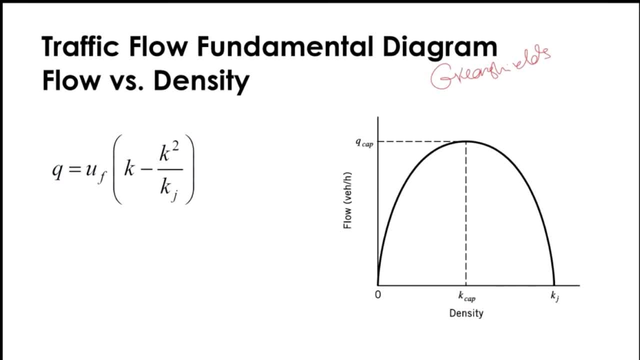 And again, as I said before, this is only an approximation of the actual relationship because if you plot real data on top of this model, we'll see that it does not necessarily match or follow real data. But again, it's a reasonable approximation. So X-axis here is density. 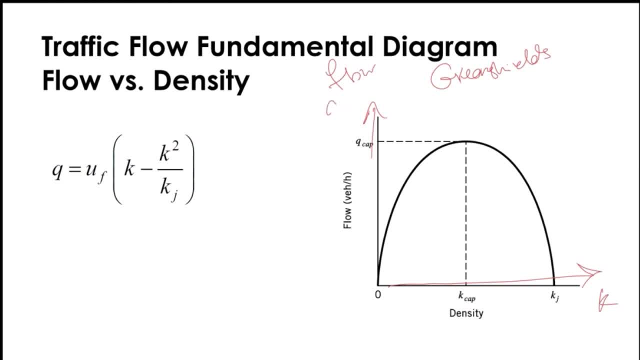 K, Y-axis is flow or Q. This is KJ. jam density, Here is maximum flow or capacity. We can also call it Q, cap or QC, And in the Green-Shields model one interesting property is that you see this KJ and this is maximum flow. 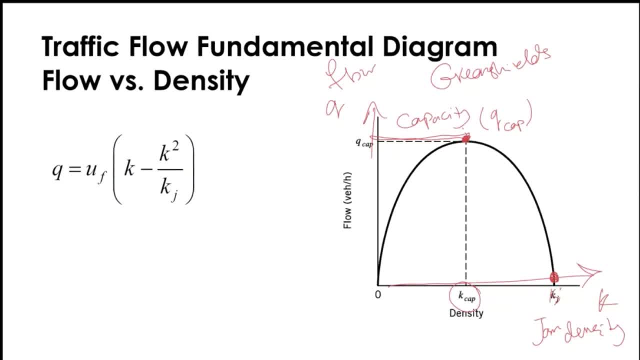 So maximum flow happens at a density that is associated with the capacity. So this K cap can be called density associated to the capacity, right, So at what density we'll have maximum flow or at what density we can reach capacity. And one of the interesting and nice properties of Green-Shields model. 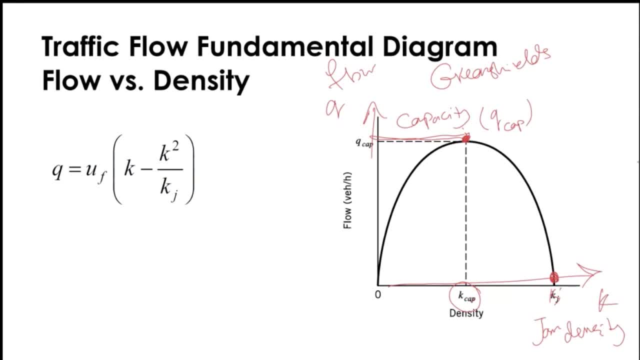 that makes it a little bit more attractive is that the density at capacity is actually equal to half of KJ. This relationship, this property, that K of capacity, density of capacity is equal to, is always half of the jam. density only holds for Green-Shields model. 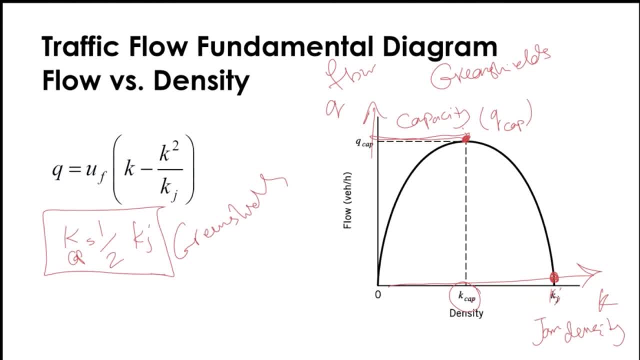 Okay, so if we are using another model, this wouldn't apply, okay, So K cap is equal to half of KJ. And again, this relationship, this equation you see here, is actually the equation for this parabolic shape curve. 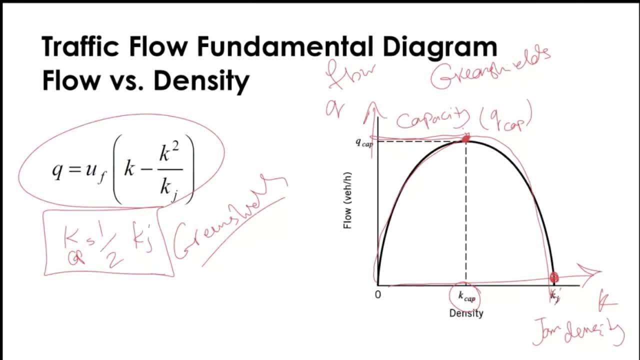 which says flow is equal to the free flow speed. So this UF again is free flow speed, Free flow speed. K is density And KJ is jam density, as I introduced before. So we'll have: Q is equal UF multiplied by K minus K, power 2 over KJ. 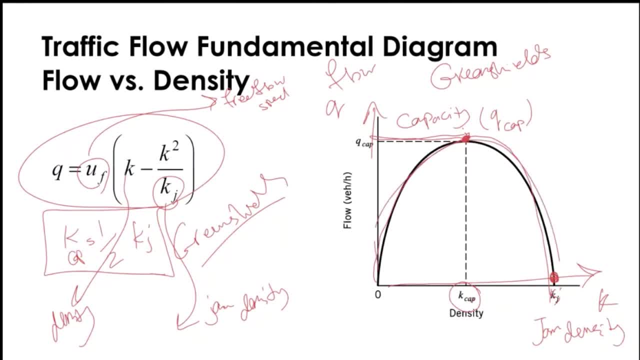 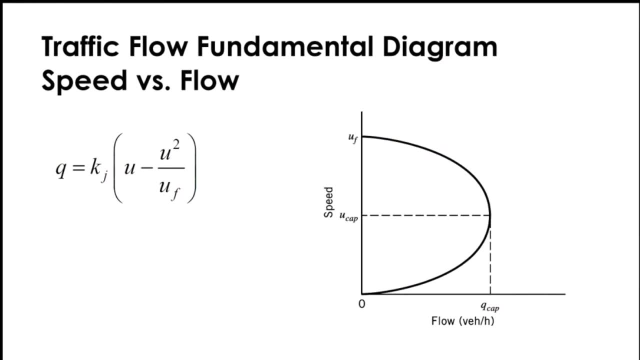 which represents this parabolic shape model. here We can also look at a speed flow relationship, right, Because all these speed flow density are related, as we covered and talked about in the previous lectures. This also looks like a parabolic type shape. 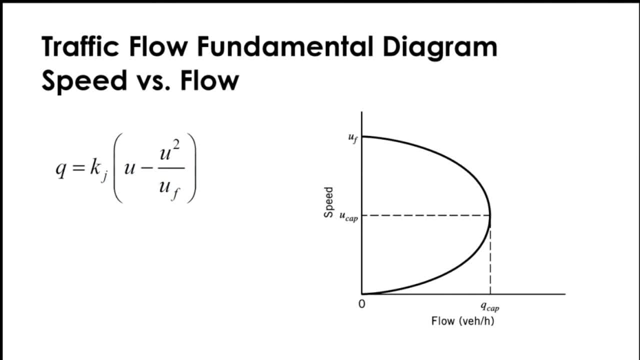 but it's not exactly parabolic, because it's actually the other way around. It's not. you know, it's not. sometimes it's not called a mathematical function because for each, for every flow, we'll have two speeds. But anyways, if we want to come up with an equation for this curve, 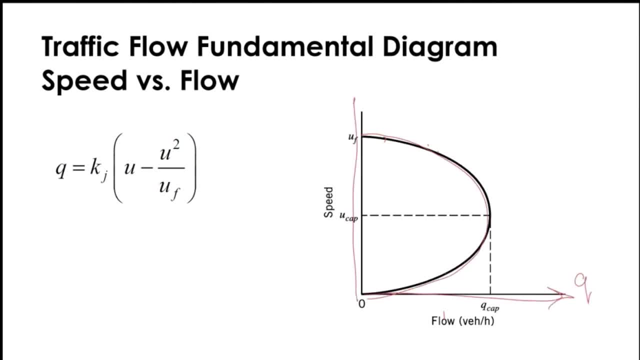 where X axis is flow and Y axis is speed, we can derive this equation saying that flow is equal to jam density multiplied by U minus U. power 2 over UF and UF is again free flow speed. So look, as long as we have KJ and UF, 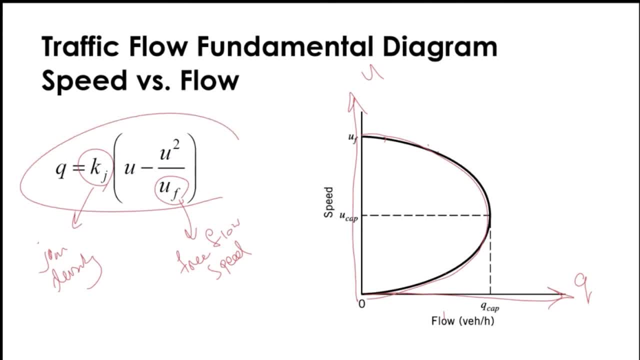 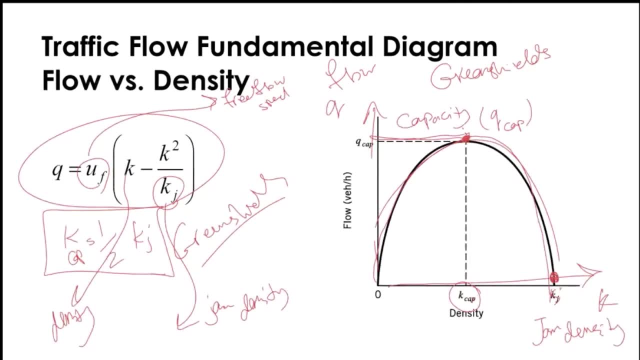 as long as we have jam density and free flow speed, we can use this equation to convert a speed to flow or flow to a speed In the previous slide. same thing: As long as we have free flow speed and jam density, we can use this equation to actually find out. 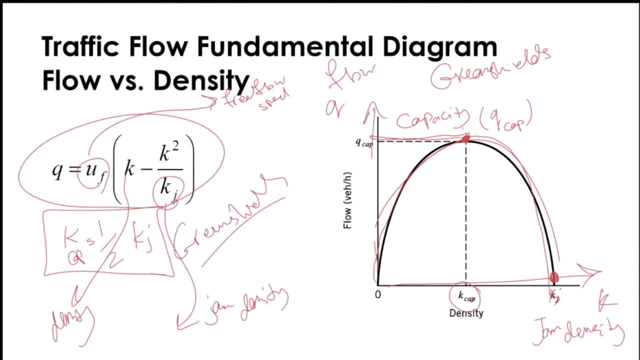 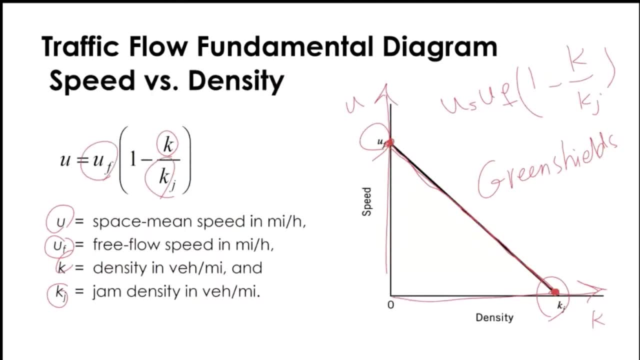 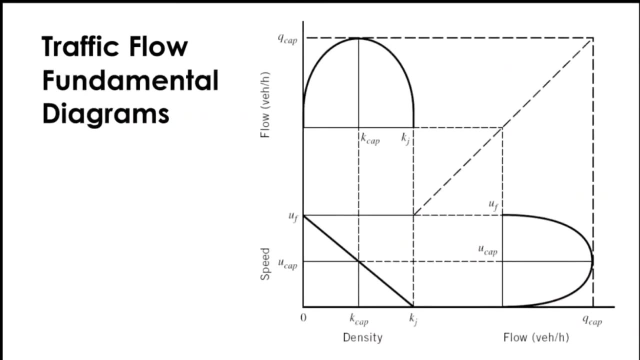 what would be the flow? if density is at whatever number, We can convert density and flow Same thing with the initial one. As long as we have free flow, speed and jam density, we can convert density to a speed. Now, if you put all these three relationships next to each other, 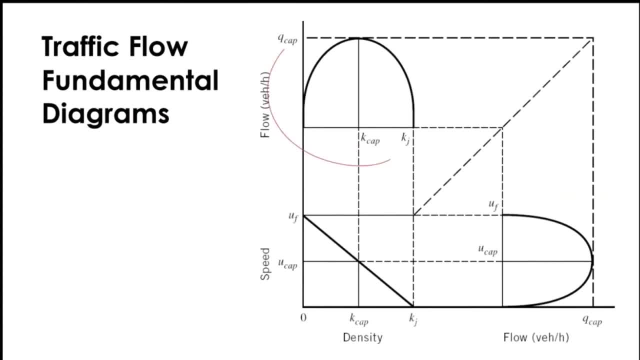 this was the density-flow relationship, this was density-speed relationship and this is flow-speed relationship. These are called traffic flow fundamental diagrams. And again, this is another very fundamental and basic modeling concept in traffic flow And it's widely used. It's very fundamental. 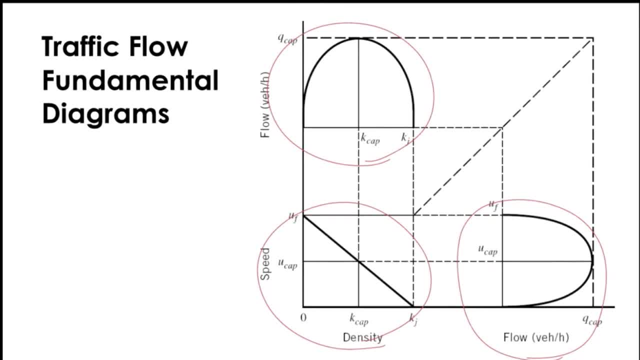 We use these relationships in many applications, when it comes to calculating speeds, when it comes to calculating flow. We use all of these models And behind some of those commercial traffic simulation softwares that you'll see in this course or you've already seen. 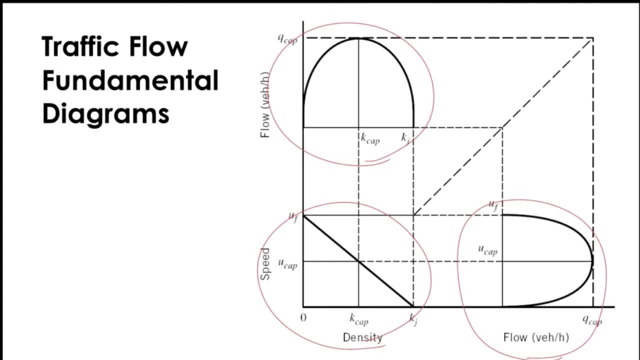 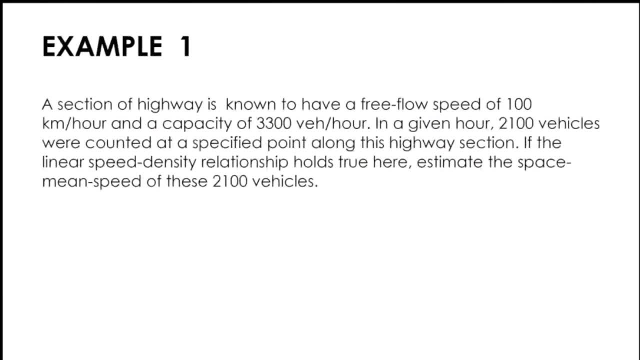 these fundamental diagrams are in play, So these are called traffic flow fundamental diagrams- the relationship between flow density, speed density and speed flow, And all of these models that I covered in this course, all of these slides were called Green-Shields model. 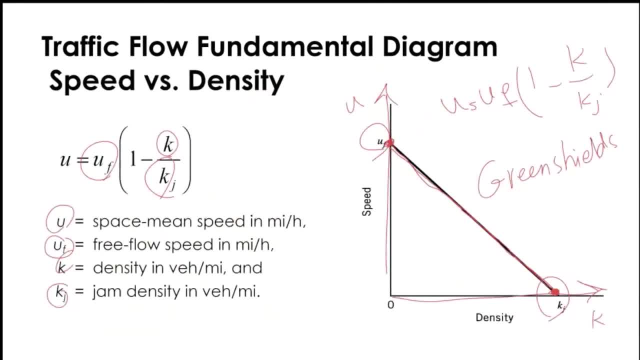 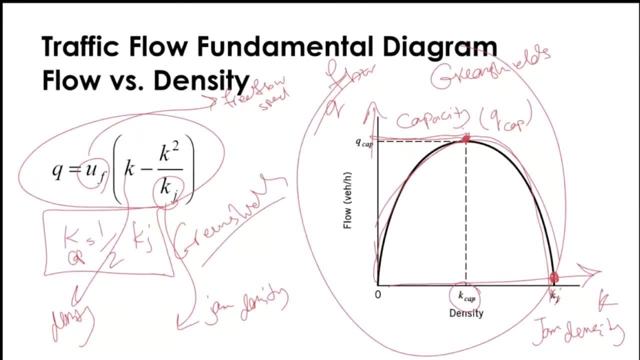 We have a couple of other models which doesn't necessarily follow the same equation. So, for example, the flow density relationship Green-Shields model assumes it's a parabolic shape, but there is another model that says this relationship is triangular or it looks different. 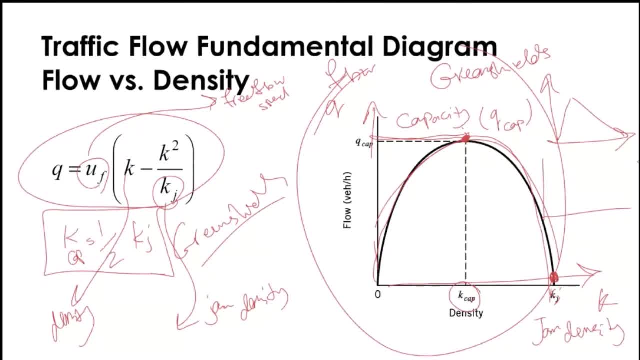 These are all single regime models, but we could have a dual regime model where, for example, we have a free flow, we have an uncongested branch and then, with some discontinuity, we have another curve on the right. So this is called a dual regime model. 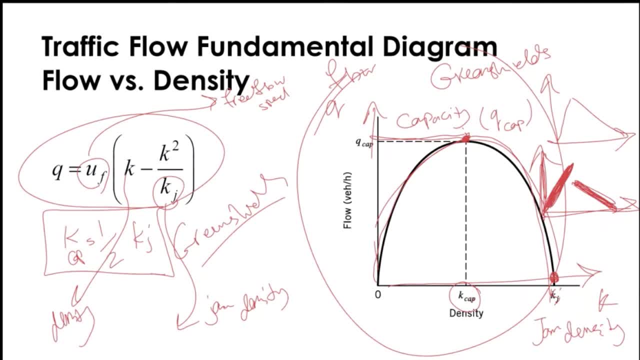 because we have this discontinuity between uncongested and congested model. But anyways, there are many different models, but here we have only focused on Green-Shields so far. Well, let's have a look at an example. Here's an example of how we can actually use. 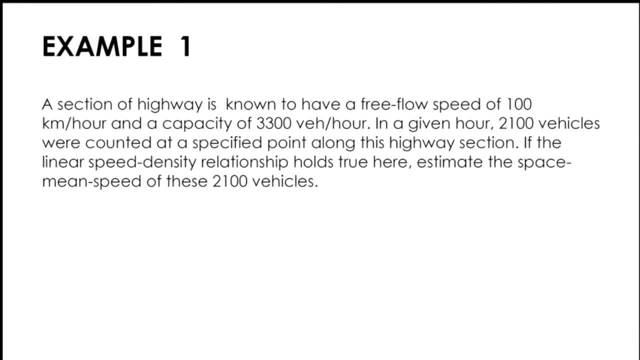 Green-Shields model in a practical problem. A section of a highway is known to have a free flow speed of 100 km per hour and a capacity of 3,300 vehicles per hour. In a given hour, 2,100 vehicles are counted. 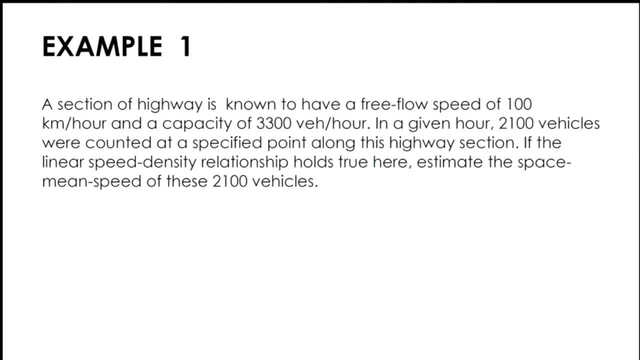 at a specific point along this highway section. If the linear speed density relationship holds true here, estimate the space mean speed of these 2,100 vehicles. So when we say if the linear speed density relationship holds true, what does this mean? This actually means we're going to go with the Green-Shields model. 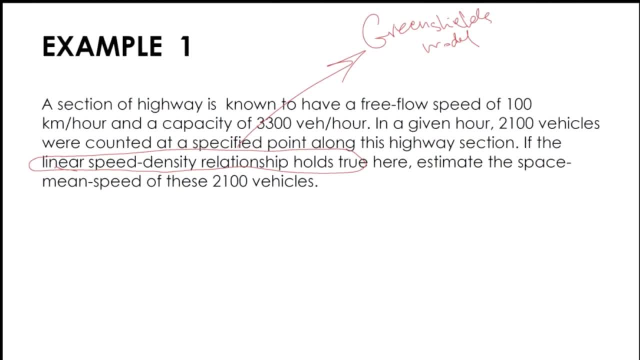 Now let's write down all the information the problem is providing us. So it says free flow speed is 100.. Make sure you also put down the units, because we want to make sure the units are consistent. Then if there is a need for converting the units to something else, 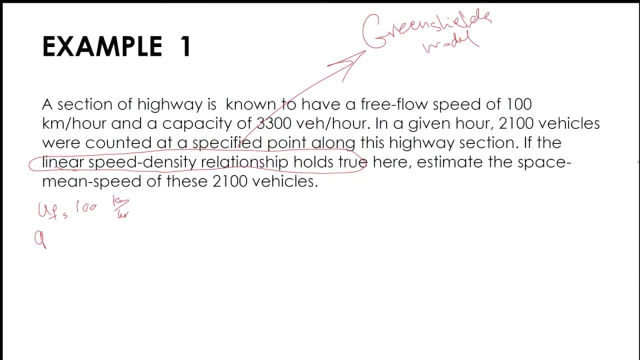 we don't want to miss that. Capacity or Q. cap is 3,300 vehicles per hour. At some point in time, Q is equal to 2,100 vehicles per hour And we want to estimate the space mean speed of these. 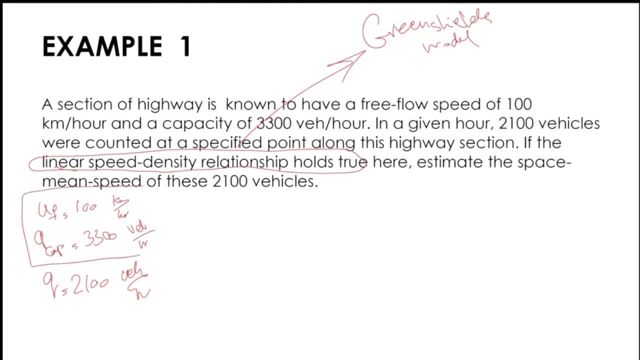 So we want to know. So we have QF and Q cap, We have the capacity and we have the free flow speed. The question is asking us: when flow is equal to 2,100 vehicles per hour, what would be the speed? 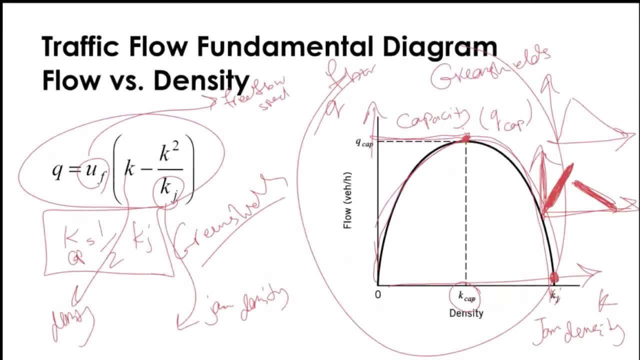 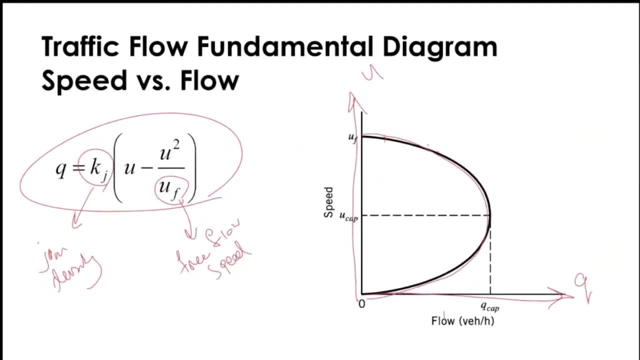 To get that, we can actually just refer back to the Green-Shields model, where we can convert speed and flow speed to flow, And we can see that we need to use this equation. to need to use this model, we actually need jam density and free flow speed. 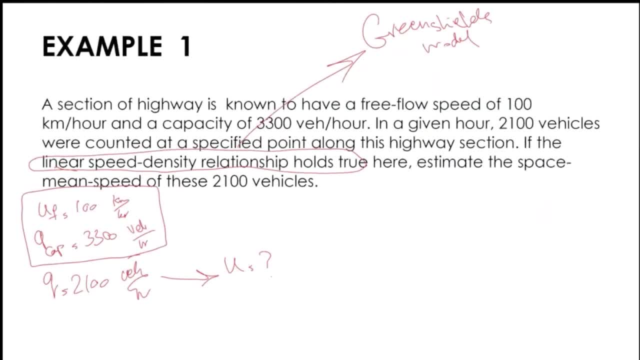 So, if I go back to my problem, I have the free flow speed but I do not have jam density, right. So let's see. So let's first write down the Green-Shields model. So, Green-Shields model, we're saying Q is equal KJ. 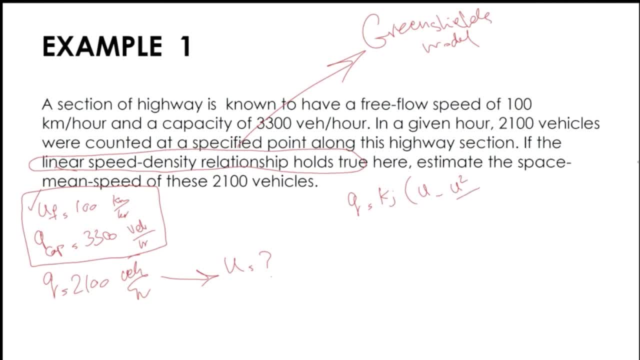 U minus U power 2 over UF. So I have UF, UF is 100, but I don't have KJ. How can I get KJ here? How can I get jam density here? So let's have a look at the. 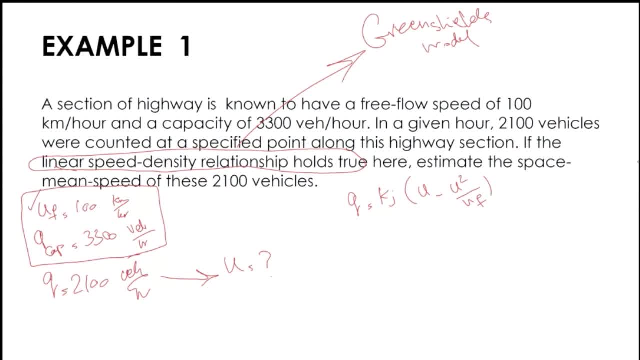 let's plot some of the fundamental diagrams here schematically. first, Let me erase this For now, So I have enough space to draw the fundamental diagrams. So if I plot the fundamental diagram relating density and flow again, we're going to go with Green-Shields model. 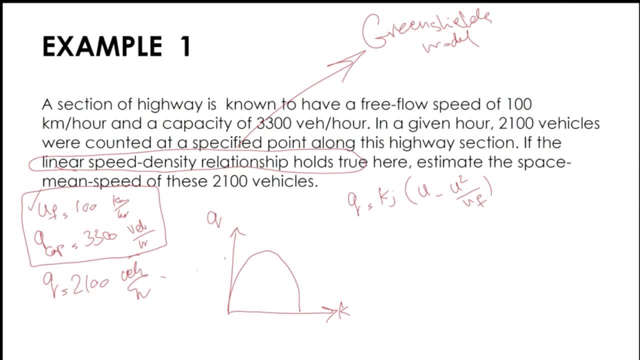 So it's a parabolic shape, right, And I know the Q cap, So this is Q cap, which is 3,300.. Let's also write K cap here and KJ. I can also draw the speed flow relationship, So this would be speed. 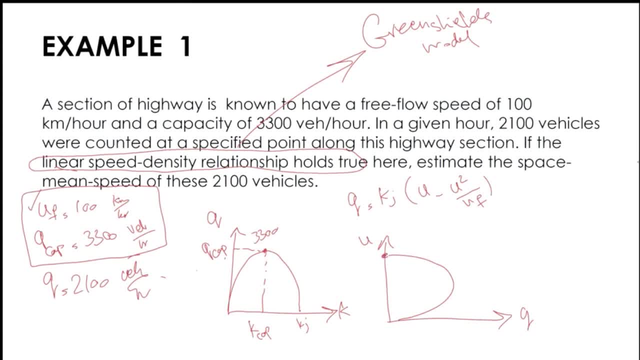 This would be flow. I have the UF, So this is UF right, Which is 100.. And again I have this Q cap, which is 3,300.. So we said in the previous slides that one of the interesting properties of Green-Shields model is that 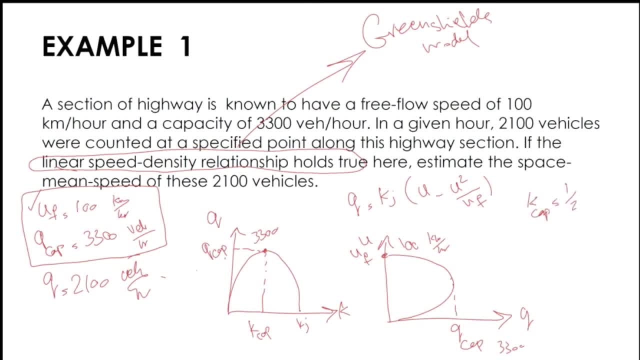 K capacity is always half of KJ. So if I somehow find this K cap and if I just multiply it by two, I would be able to get KJ right. But how can I get K cap here? So another interesting property of the Green-Shields that can be seen on this UF. 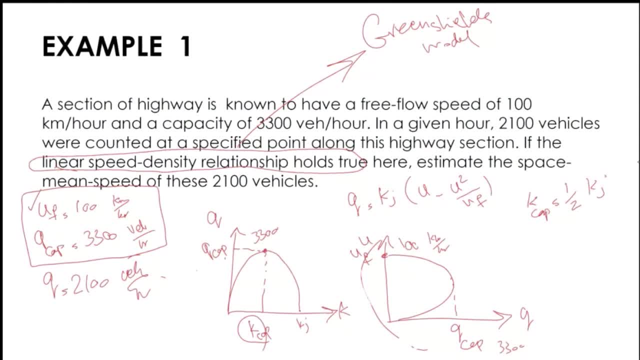 which can be seen on the right diagram here, is that the speed associated with the capacity- let's also call it U cap- is also half of UF. So the speed at capacity in this case would be 50 km per hour. right, 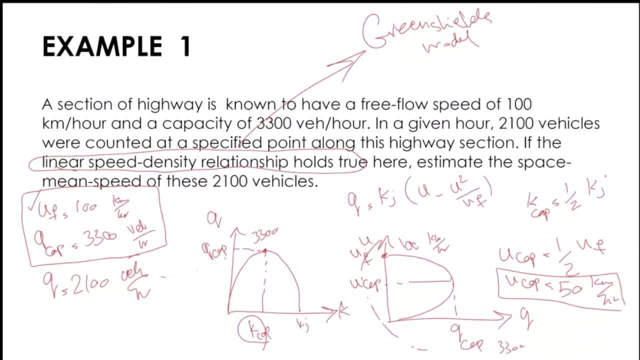 Because it's half of this, the free flow speed. Again, I want to highlight here these K cap- equal half of KJ and U cap- equal half of free flow speed- only holds true when we're working with Green-Shields model. If you're working in another model, this may not necessarily hold true. 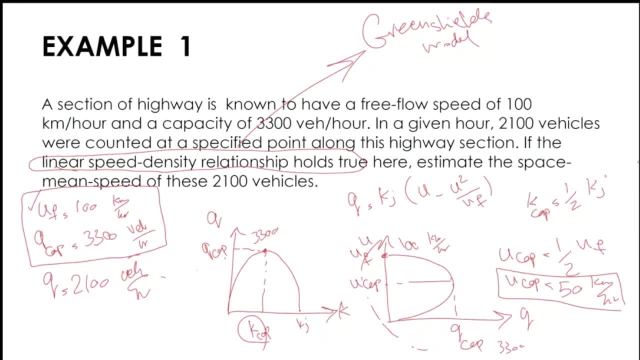 So now that I have the speed at capacity and I have the actual Q cap, I can get K cap right If I use the traffic flow fundamental identity which is Q equal KU right. So if I want to get K cap, 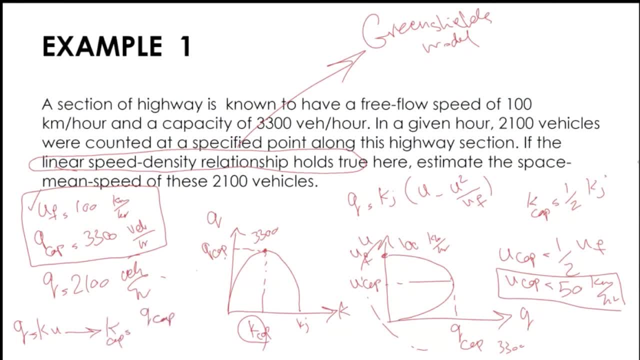 I just need to say the flow at capacity, or capacity equal to the speed at capacity. So I had 3,300 over 50. And if I calculate that I'd get K cap would be equal to 66. So that would be vehicle per kilometer. 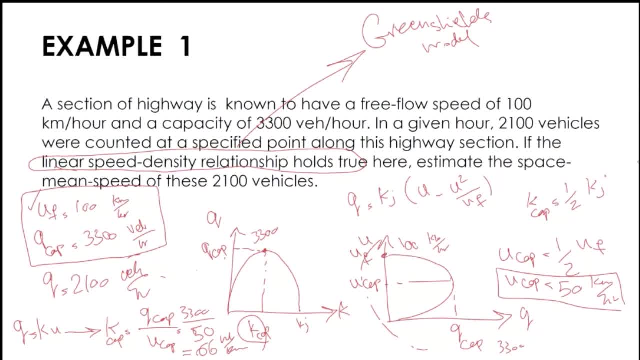 So that's my K cap, And again because K cap is equal to half of KJ in this case, so KJ would be 66 multiplied by 2. It would be 132 vehicle per kilometer. So I somehow found jam density. 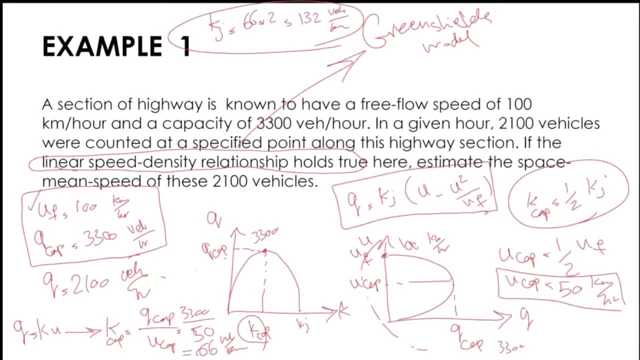 Now that I have jam density, I can actually use the Green-Shields model to actually calculate the speed when flow is equal to 1,200.. So if I write this Green-Shields model again here, so it would be: Q is equal to 132. 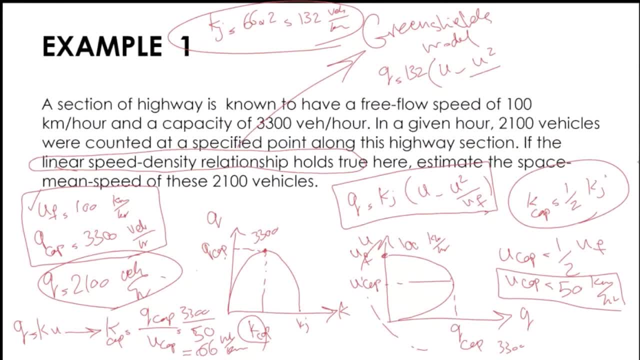 U minus U power 2. And the free flow speed was 100.. So I have this relationship now And the question is asking: estimate the speed when flow is equal to 1,100.. So if I just replace this Q here with 2,100,. 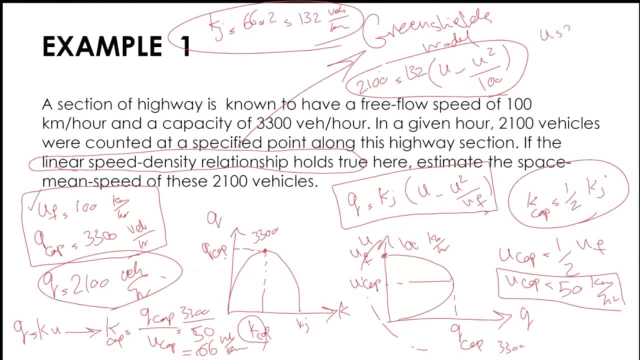 and if I solve this equation I would be able to get U right. So if I want to draw that on the fundamental diagram, so 2,100 is somewhere here. right, So 2,100.. But what is interesting here is: 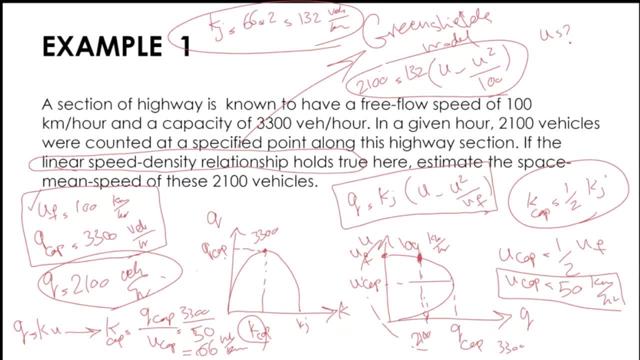 because of this parabolic type shape relationship. if we solve this equation, we're actually going to find out two values for this speed. You see, For the flow equal to 2,100, I can either find this speed or this speed. 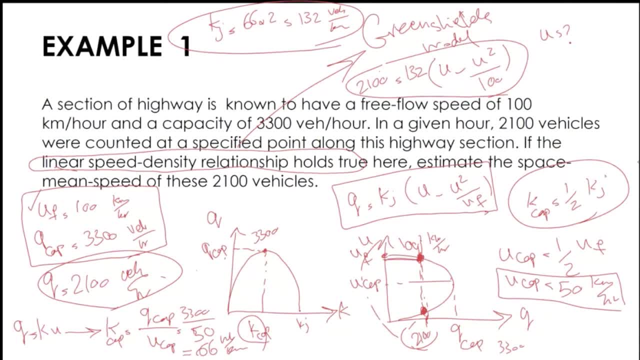 So one of them is in the uncongested regime, The other one is the congested regime. So how does it? I mean, how can we interpret this? So look, if you are in the uncongested regime, the road is not very crowded. 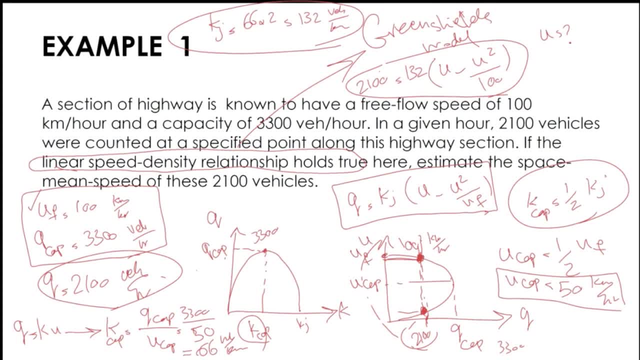 The flow is relatively small, lower than capacity, So speeds are going to be high. So if I find a speed, if I find this point, then I solve this equation. one speed that I get will be on the uncongested branch. 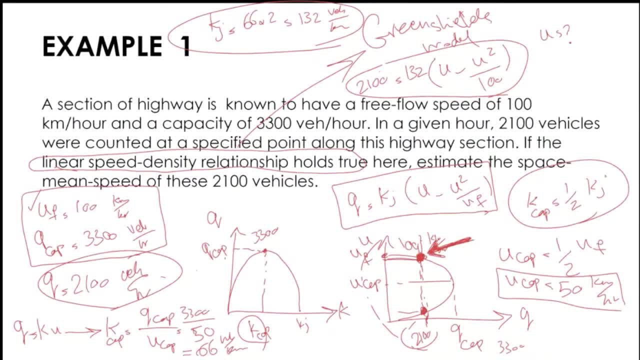 But when the road is congested there's too many traffic. So the flow is low, not because there isn't enough cars on the road. The flow is low, lower than capacity, because there is congestion on the road. So in the first point, on the uncongested branch, 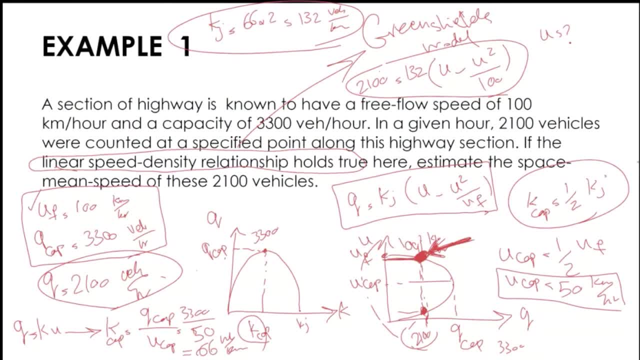 the flow is low but the speed is high because it's uncongested. But the other point, on the bottom, the flow is lower than capacity because it's congested. There's enough car, but there's a queue on the, there's a queue on the road and a speed is low. 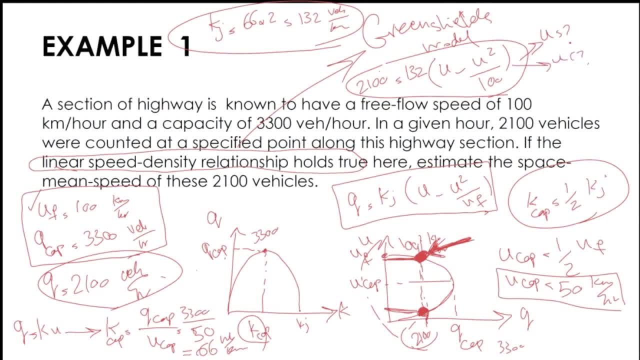 So I will get two values for you, if I find this equation, And one of them. both of them are correct. One of them relates to: if flow is 2,100 and if we are in the uncongested regime, we'll have the higher speed. 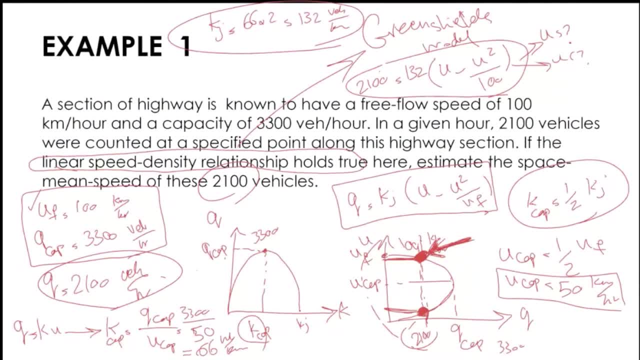 If we are in the, if we are in the congested regime- congested regime- we'll find the lower, the lower speed would be the correct answer. So let's actually try to find the answer to this equation. We want to actually find the root of this parabolic shape. 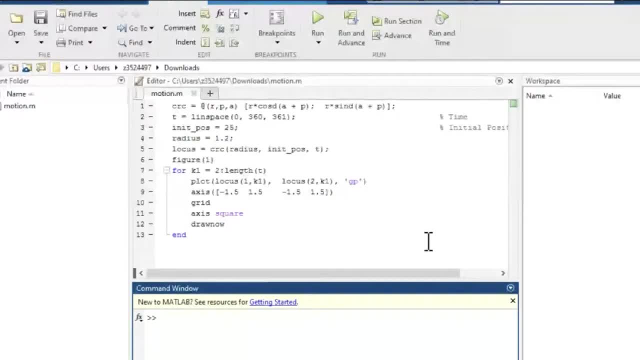 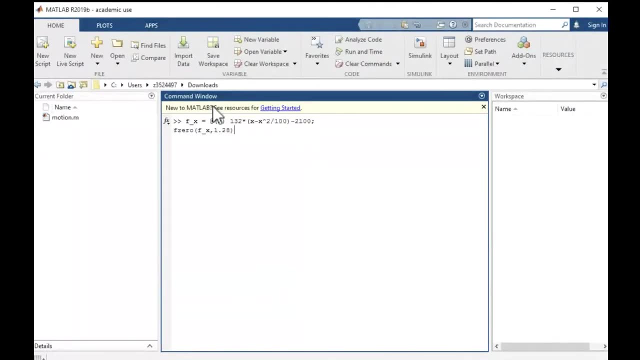 polynomial equation. So if I go to MATLAB, okay, so here let me get rid of this tab. So here, to find the root, I need to define a function, And my function is actually my Green Shields model, which was KJ: multiply U minus U power, two over free flow speed minus 2,100. 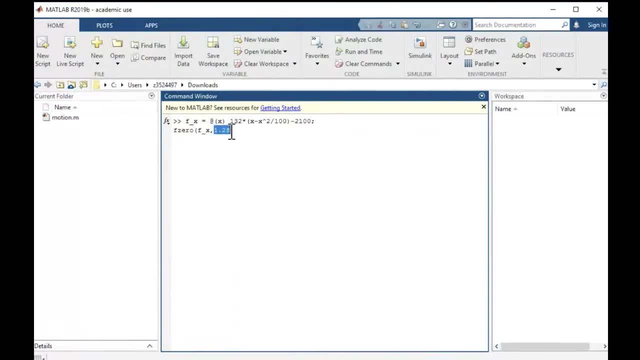 And if I find the root of this equation, I can use F, zero, and I need to give it an initial answer, right? For example, I start with zero as the initial answer. Let's see what it gives me. So one U would be equal. 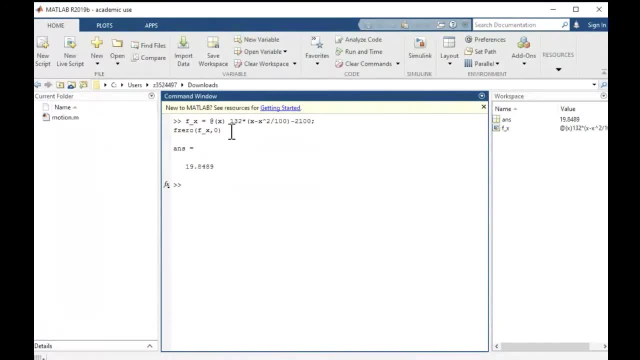 one speed would be equal to 19.85 kilometer per hour. And if I change the, if I change the initial answer to actually find the other root of the equation? for example, if I give the initial answer 200, it will find the other root. 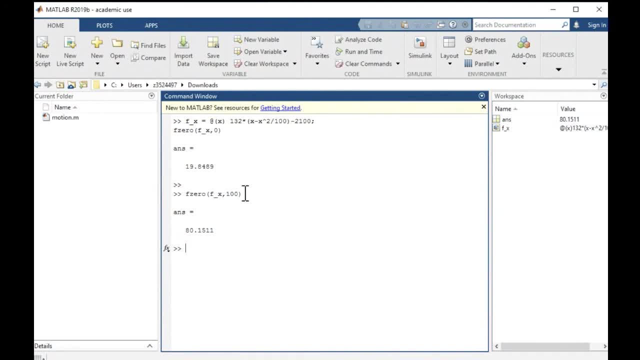 which is equal to 80.15 kilometer per hour. So you see, I get one speed which is low and one speed which is high. So obviously this, this speed equal to 19.85, is from the congested regime. 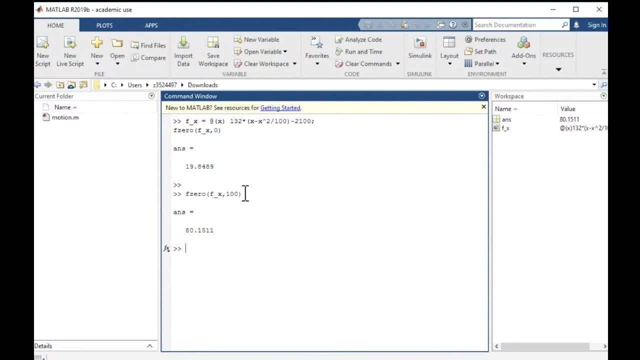 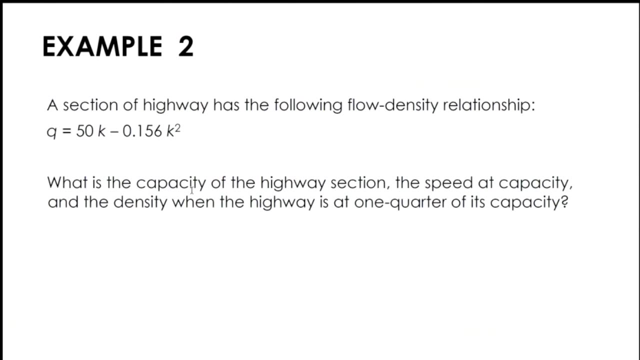 When the flow was equal to 2,100,, while the speed equal to 80, is coming from the uncongested regime and the flow was still 2,100.. Let's have a look at a second example. Imagine a section of highway. 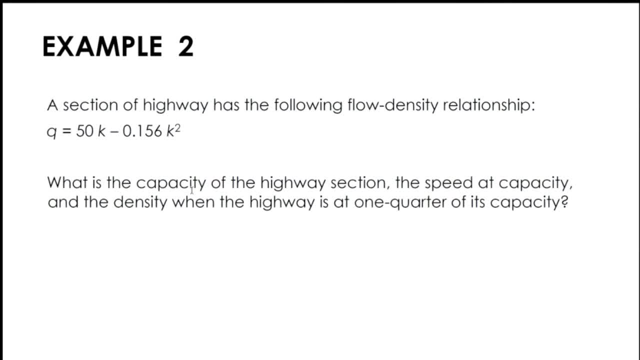 that has the following flow density relationship: What is the capacity of the highway section, The speed at capacity and the density when the highway is at one quarter of its capacity? So this is again a parabolic relationship, right? So if I draw the traffic flow fundamental diagram, 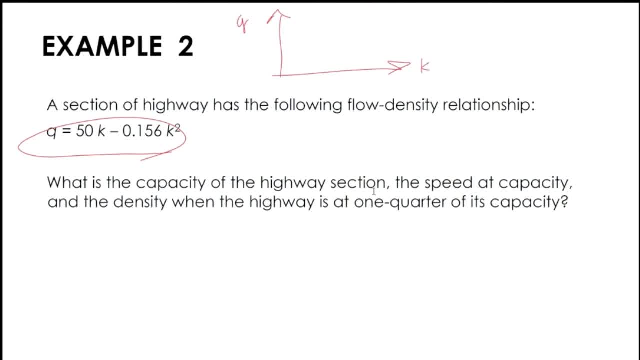 I have K here, I have Q here. I have a parabolic curve here, I have KJ, I have jam density, I have capacity here, I have K at capacity, et cetera. So the question is asking us. 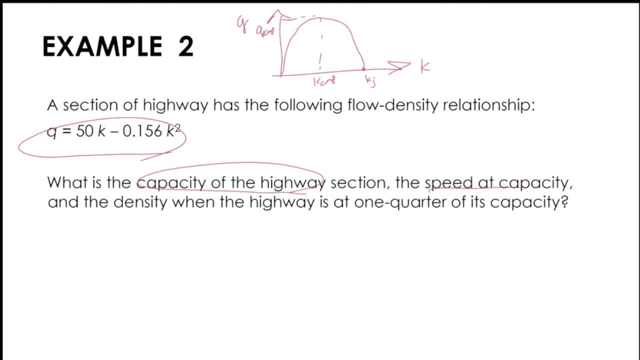 what is the capacity of the highway section, What is the speed at capacity, What is the den and the density when the highway is at one quarter of its capacity? So how can I, how can I answer this question? So, first of all, 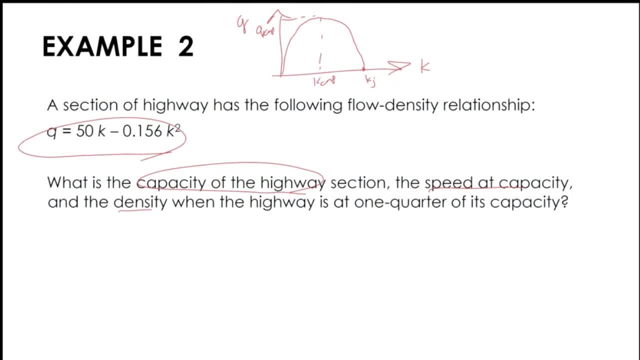 how can I get the capacity here, If I have the Green Shields model, if I have this parabolic relationship, if I want to get that maximum point? so you see, capacity is at the maximum point of this curve. So if I want to get that maximum point, 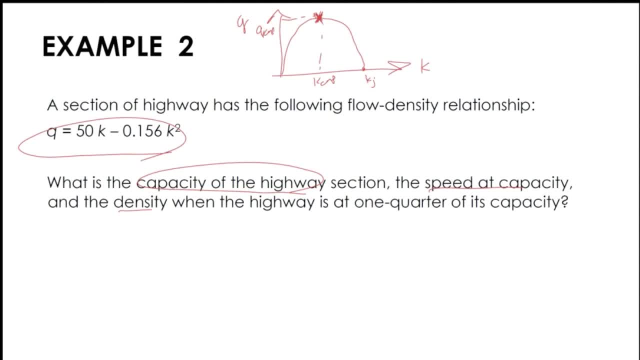 what should I do? I can take the derivative of this equation, make it equal to zero and I will be able to get that maximum point. So if I go with DQ over DK and make it equal to zero, I would be able to get that capacity. 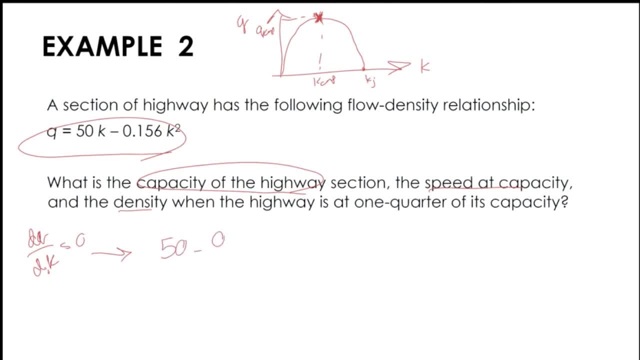 So that would give me 50 minus six power two, sorry, not power two. multiply by two equal to zero, And this will give me the density that I need, the density at capacity. So if I solve that, let me quickly calculate that. 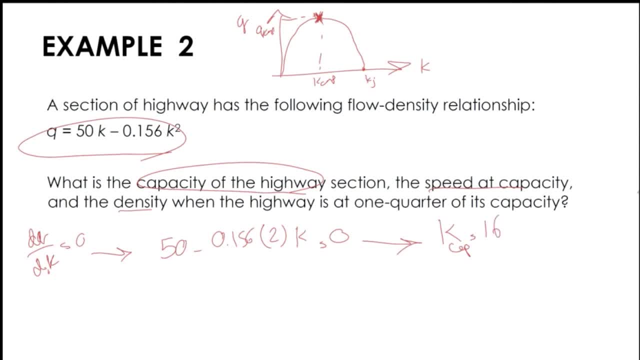 So K would be equal to one sixty point point two, six, if I haven't made any mistake in my calculation. So that's K cap, the density associated to the capacity. But the question is asking for the capacity itself actually. So I need to put this K cap into the 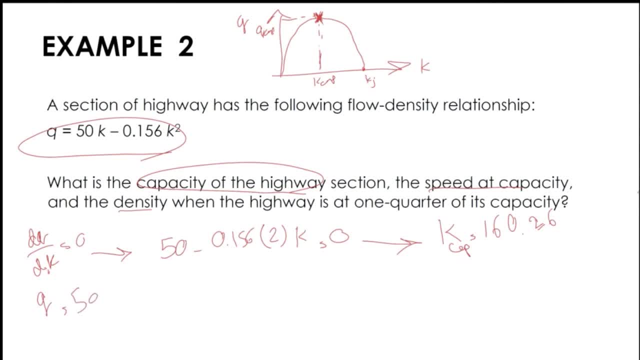 back to the equation and calculate the flow. So flow would be 50, one sixty point twenty six, minus one five six one sixty point twenty six power two. Okay, calculate that That would be equal to. so Q cap would be equal to four thousand six point four. 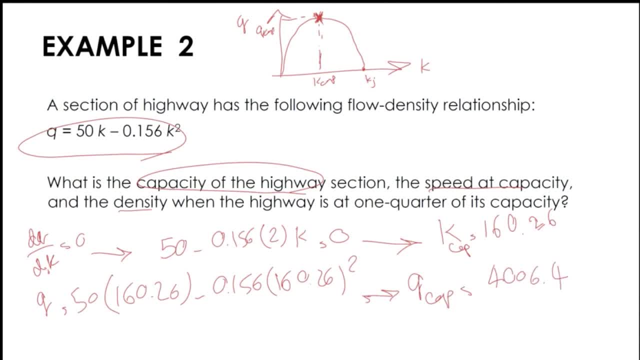 if I haven't made again any mistake here. So that's the capacity. The question is also asking us about the speed at capacity. I have the density at capacity, I have the flow at capacity, so I can easily use the traffic flow. fundamental. 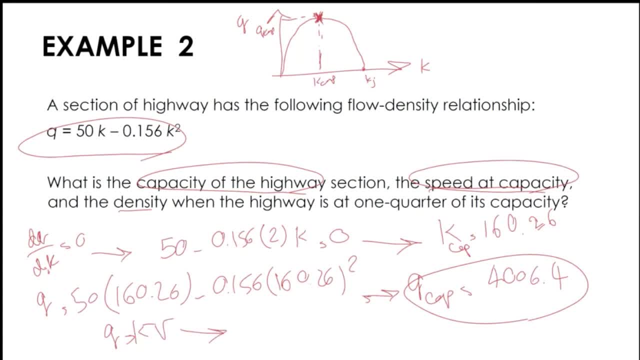 identity: Q equal KV to calculate the speed at capacity. So speed at capacity would be Q over K And if I calculate that that would be equal to twenty five. So I have the speed and the question at the end is asking: find out the density. 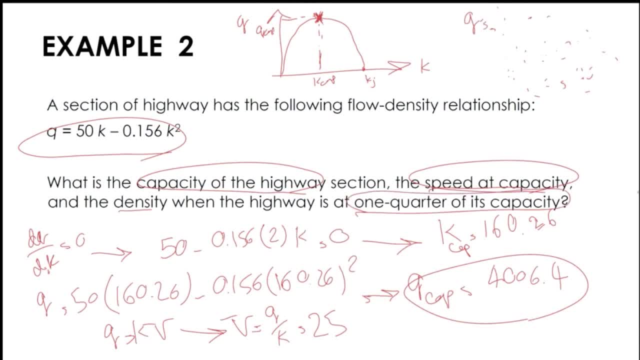 even the highway is at one quarter of its capacity. So Q is equal to one fourth of Q cap. So it would be one fourth of four thousand six point four. So if I calculate that that would be, so Q equal to one thousand one point six. 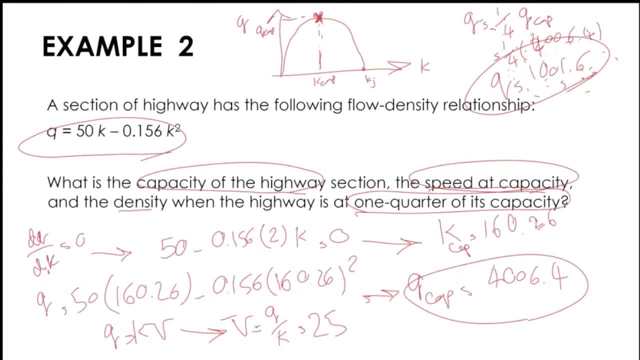 So that's the flow At one quarter of its capacity. we want to know what is density, So we just need to put this Q into the Green Shields equation, So it would be one thousand one point six is equal to fifty K minus one. five. six K power two. 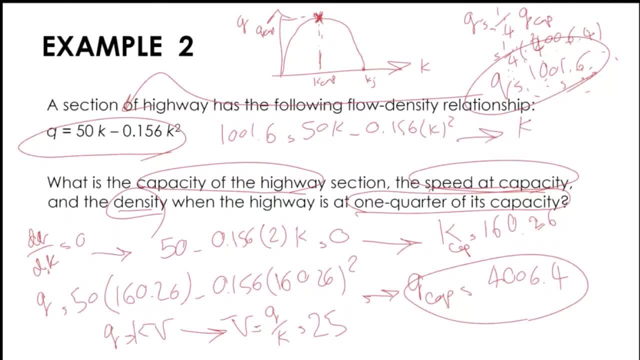 And if I find the root of this equation, I'll get the K that I need. And again, I will get two Ks. right, I will get two values for density, because this would be the one thousand one point six, So I would get one density here. 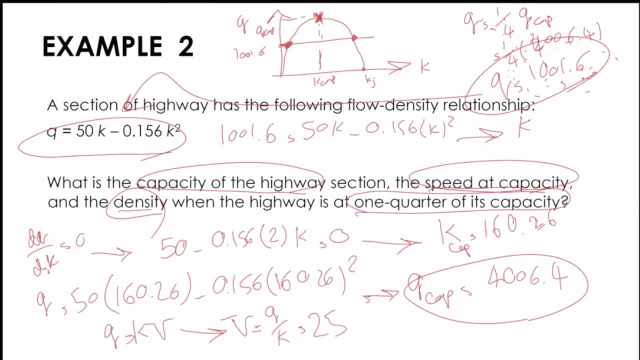 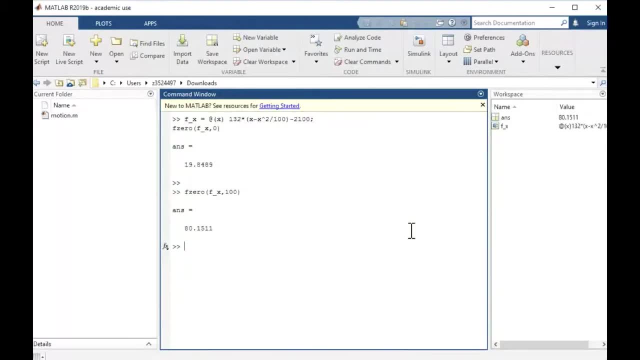 and one density here. So let's do that also in MATLAB again to find the root of this equation. If I write it down here, I want to find the root of this equation. So I say F, X is equal to at sine X. 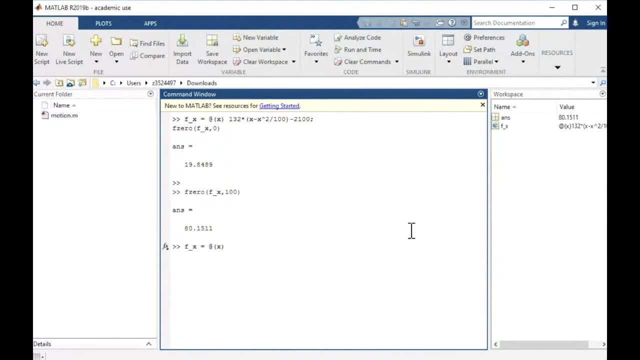 which is I'm defining the variable in my equation. So it would be fifty X minus one, five, six X power, two minus one thousand one point six. So that's my function And if I want to find its root, if I give zero as the initial, 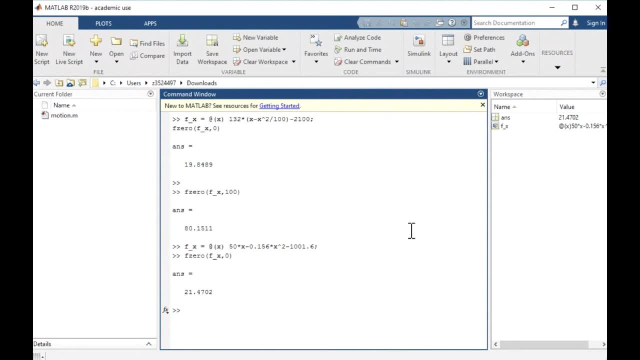 guess for the solution. so one K. So the first solution would be: density is equal to twenty one point four, seven, And if I give it another initial guess, over two hundred. Yes. So the other one would be: K is equal to two, nine, nine zero four, two, six. 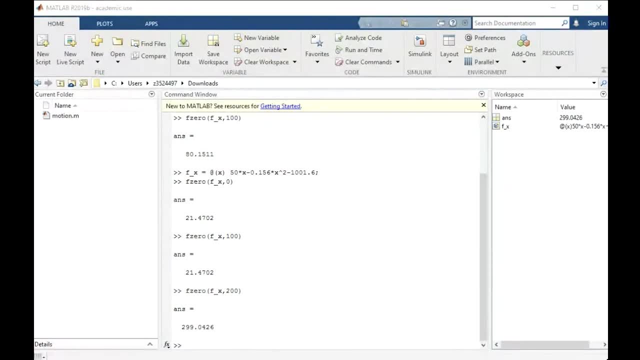 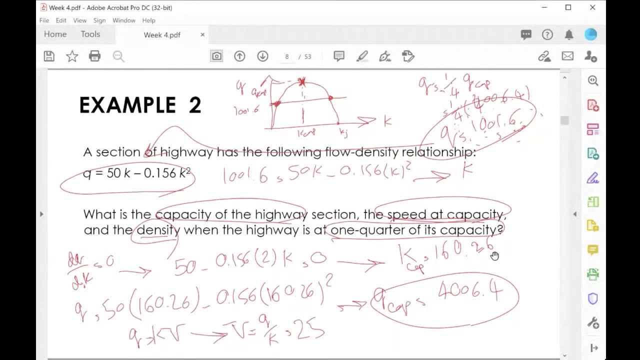 If I go back to my slides. So what is jam density here? If the density at capacity is one sixty point two six, jam density would be double than the K at capacity, right? So we just need to multiply this one six, one one sixty by one sixty.